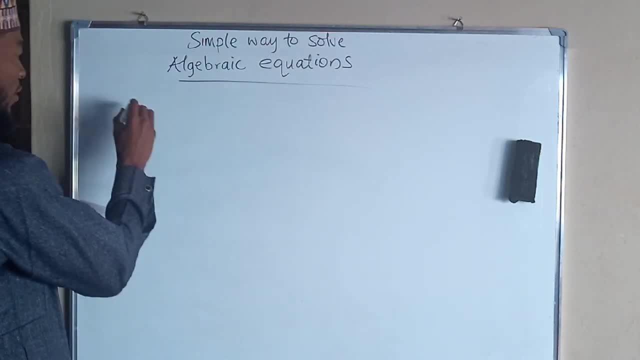 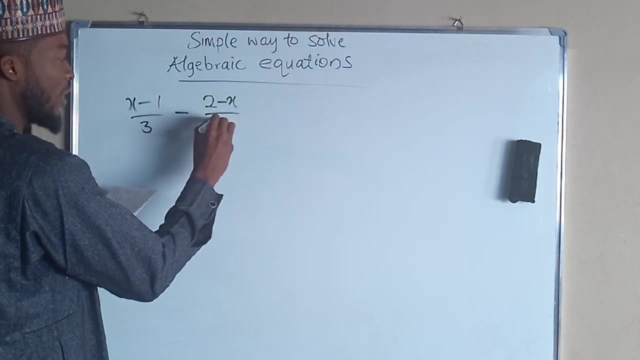 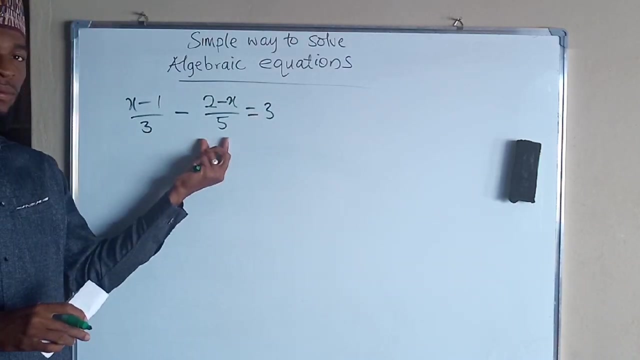 best way. So first you have an equation like this that says you should simplify: x minus 1 divided by 3 minus 2 minus x divided by 5 equals to 3.. Now we have denominators 3 and 5.. Please, before going further, please try as much as. 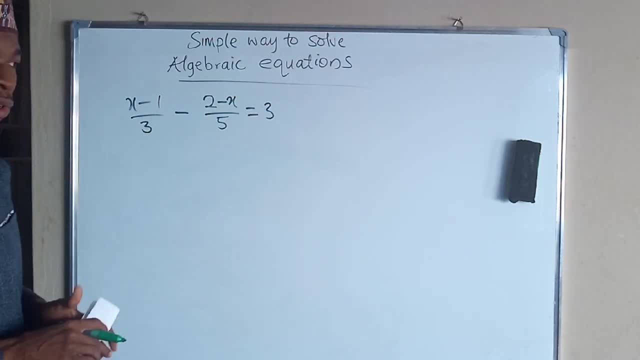 you can to eliminate them out. How do we do that? By multiplying each term by the LCM of these denominators, and the LCM of 3 under 5 is 15.. So we are going to multiply each term by 15, so that we have 15 multiplied by x minus 1 divided by 3. 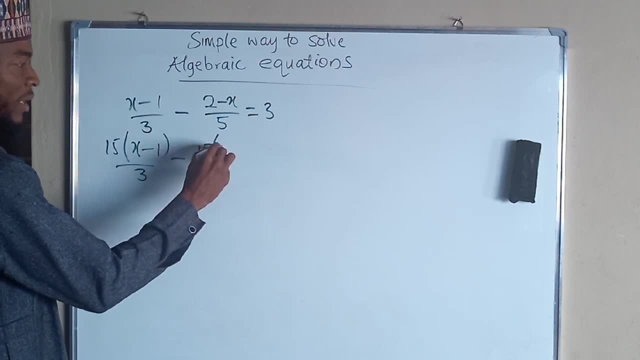 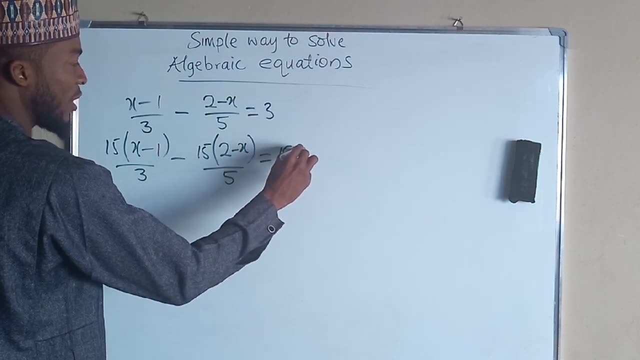 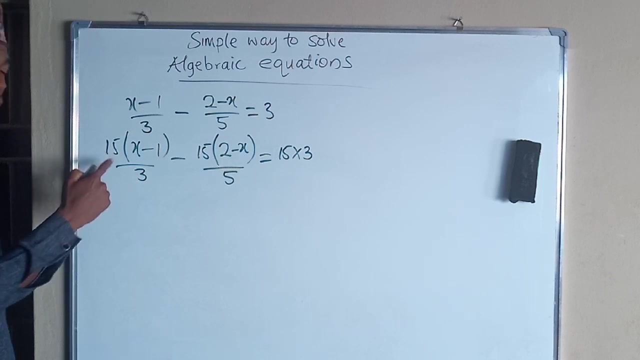 minus 15, in the bracket of 2 minus x By 5, all of this equals to 15 times 3.. We go further. We know that 3 can go into 15 five times. Then that 5 we are going to multiply x minus 1.. So 5 times x is going. 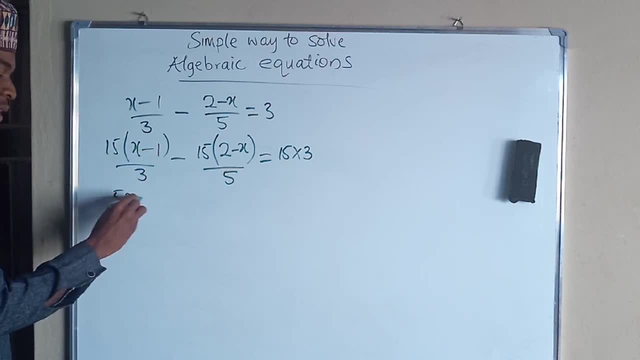 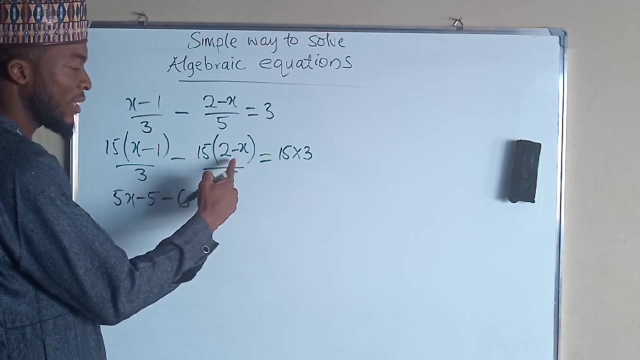 to give you 5x, Then 5 times negative 1 is negative 5. And here you know that 5 can go into 15 three times. Then negative 3 times 2 is what Negative 6.. Then negative 3 times negative x is going. 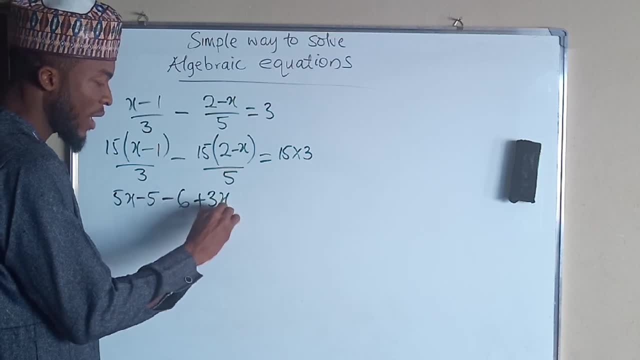 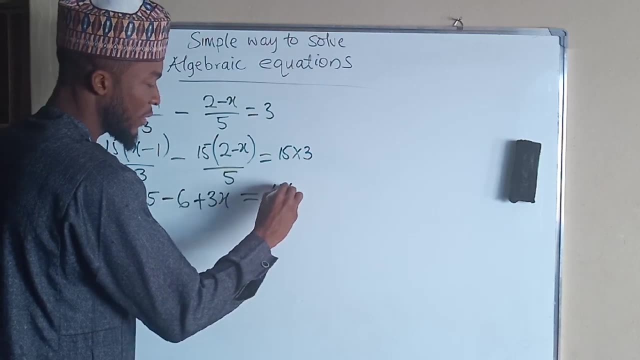 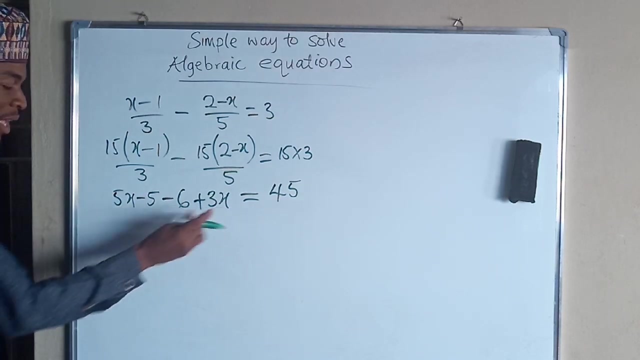 to give you positive 3x, And this is equal to 15 times 3,, which is 45.. 45. Now we know that 5x plus 3x is going to give us 8x. Negative 5 minus 6 is going to give us negative 11. And this is equal to 45. Now we are going.